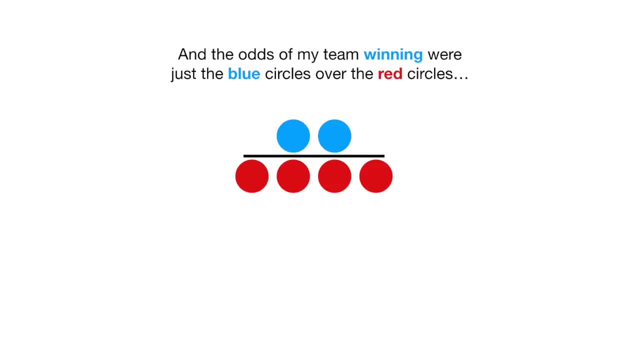 And the odds of my team winning were just the blue circles over the red circles. Alternatively, we could just use numbers to represent the odds And when we do the math we see the odds of winning are 0.5.. The cliffhanger came when I said that, even though the odds are a ratio, it's not what people mean when they say odds ratio. 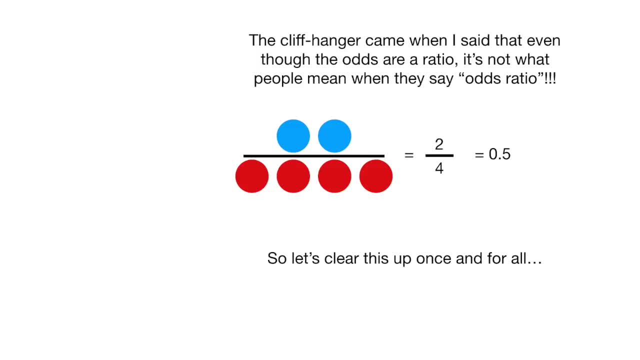 So let's clear this up once and for all. When people say odds ratio, they're talking about a ratio of the odds. So let's clear this up once and for all. When people say odds ratio, they're talking about a ratio of the odds. 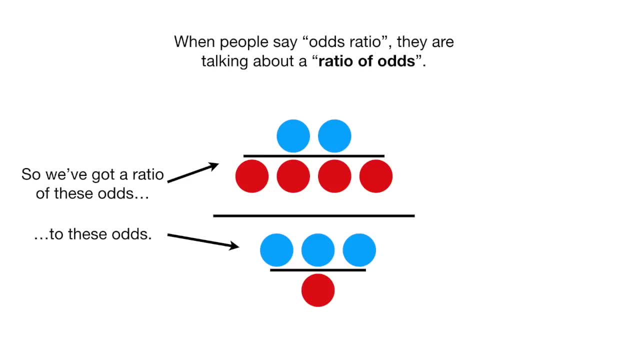 So we've got a ratio of these odds to these odds. So we've got a ratio of these odds to these odds. Doing the math gives us 2 divided by 4 over 3 divided by 1.. Doing the math gives us 2 divided by 4 over 3 divided by 1.. 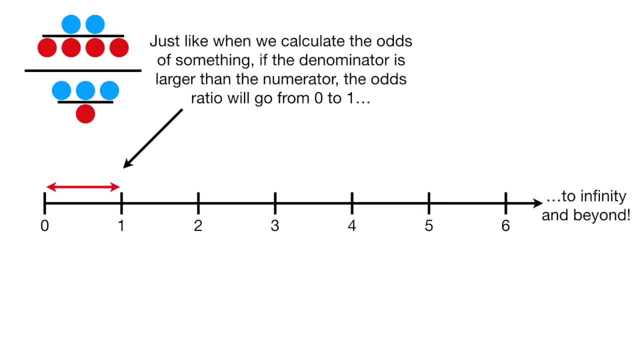 And that gives us 0.17.. Just like when we calculate the odds of something, if the denominator is larger than the numerator, the odds ratio will go from zero to one. The odds ratio will go from zero to one. And if the numerator is larger than the numerator, 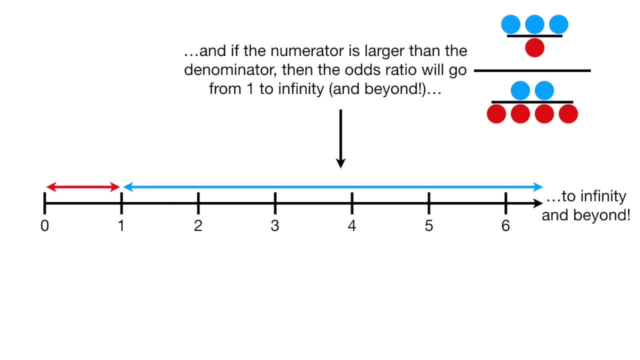 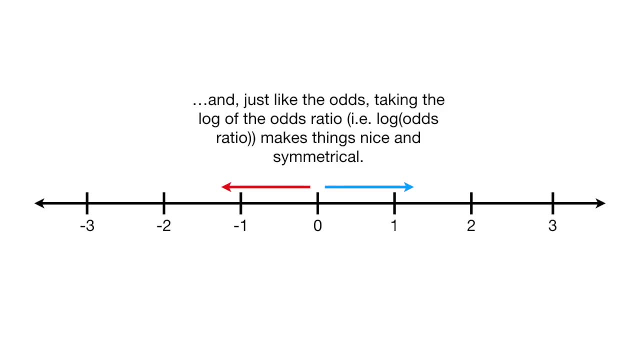 larger than the denominator, then the odds ratio will go from 1 to infinity and beyond. And just like the odds taking the log of the odds ratio makes things nice and symmetrical. For example, if the odds ratio is 2 divided by 4 over 3 divided by 1, then the log of 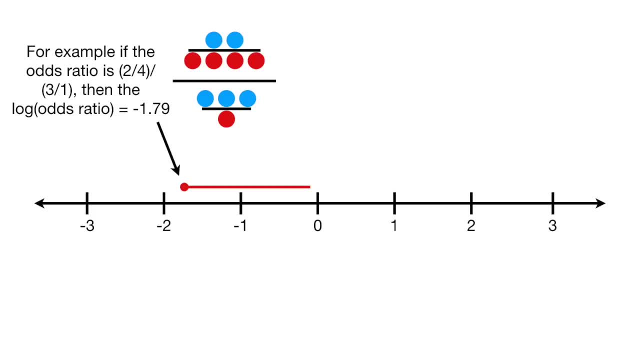 the odds ratio equals negative 1.79.. And if the odds ratio is the opposite, it's 3 to 1 over 2 to 4, then the log of the odds ratio is the positive version. It equals 1.79.. 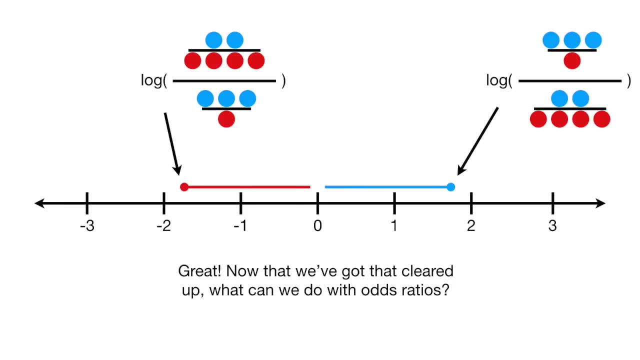 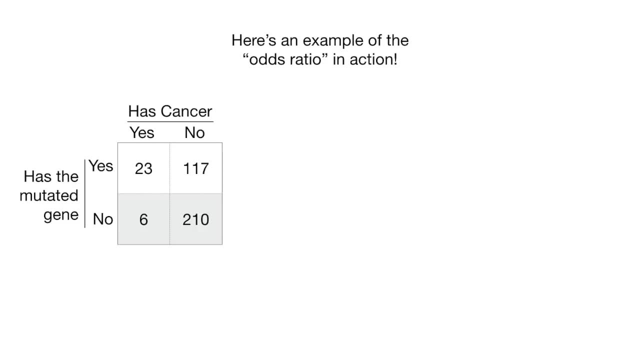 Great. Now that we've got that cleared up, what can we do with odds ratios? Here's an example of the odds ratio in action. We've got a bunch of people, 356 to be exact. 29 of these people have cancer. 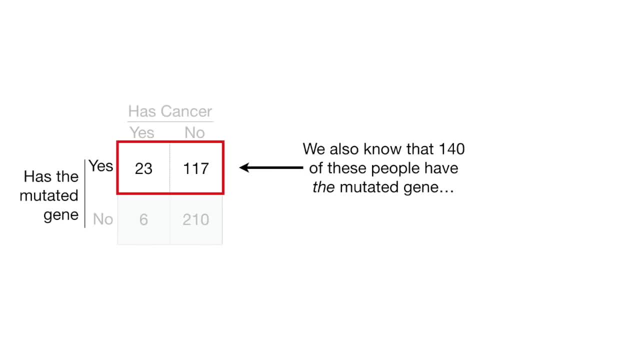 And 327 do not. We also know that 140 of these people have the mutated gene- I'm just going to let you imagine which gene I'm talking about here- And 216 people do not have the mutated gene. We can use an odds ratio to determine if there's a relationship between these two people. 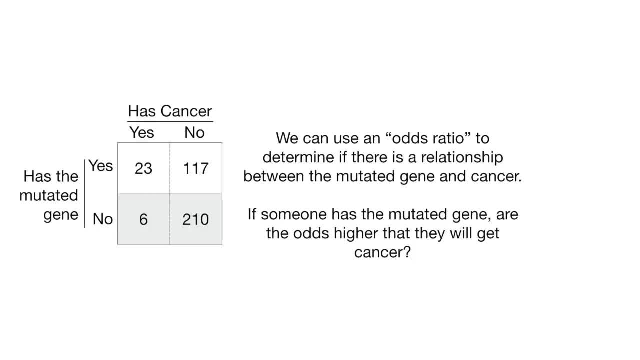 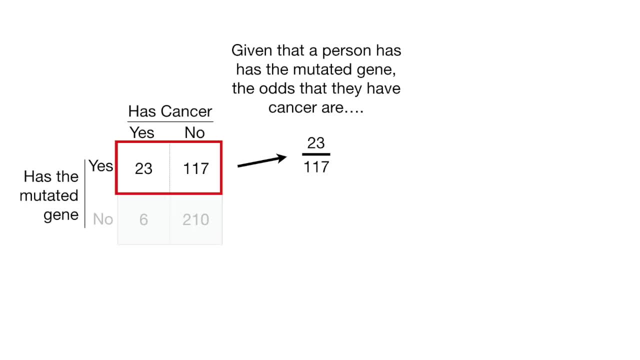 Here's what we're going to do: We're going to divide the odds ratio between the mutated gene and cancer. If someone has the mutated gene, are the odds higher that they will get cancer. Given that a person has the mutated gene, the odds that they have cancer are 23 to 117.. 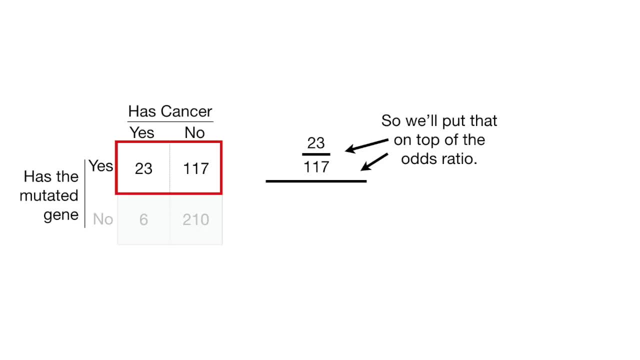 So we'll put that on top of the odds ratio. And, given that a person does not have the mutated gene, the odds that they have cancer are 6 to 210.. Great, So we'll put that on the bottom of the odds ratio. 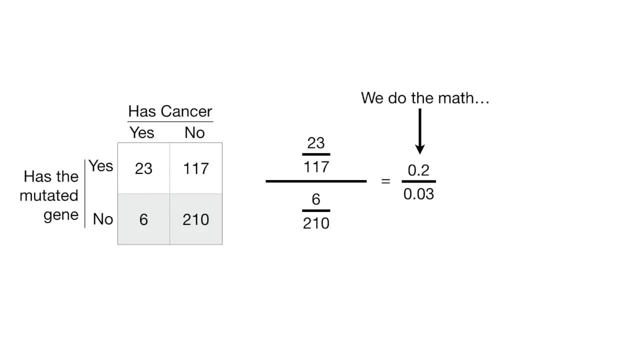 Here's our odds ratio. We do the math And the odds ratio tells us that the odds are 6.88 times greater that someone with the mutated gene will also have cancer, And the log of the odds ratio is 1.93.. 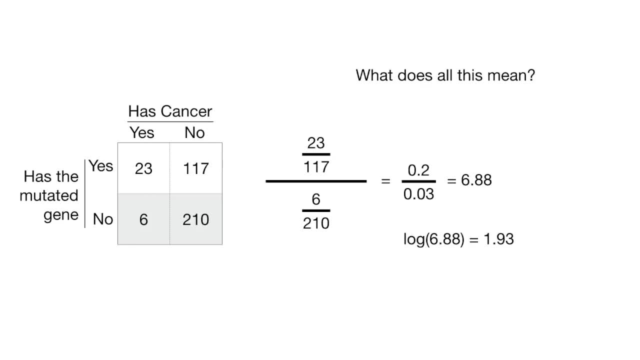 Small bam. What does all this mean? The odds ratio and the log of the odds ratio are like R-squared. They indicate a relationship between two things, In this case a relationship between the mutated gene and cancer. And, just like R-squared, the values correspond to effect size. 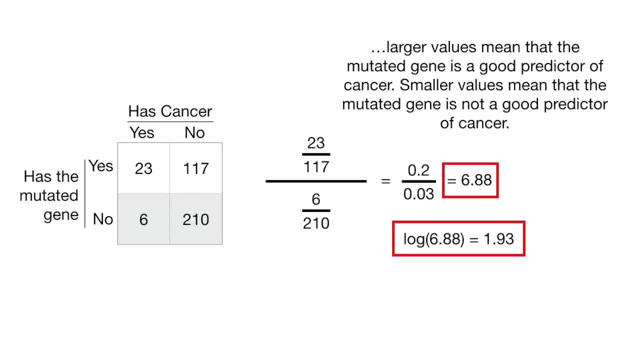 Larger values mean the mutated gene is a good predictor of cancer. Smaller values mean that the mutated gene is a good predictor of cancer. Larger values mean that the mutated gene is not a good predictor of cancer. Bam, However, just like R-squared, we need to know if this relationship is statistically significant. 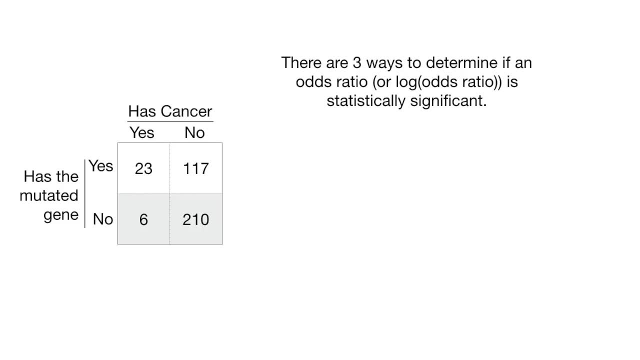 So let's do it. There are three ways to determine if an odds ratio or log of an odds ratio is statistically significant. Fisher's Exact Test. Fisher's Exact Test. One super annoying thing is that there is no general contensis on which method is best. 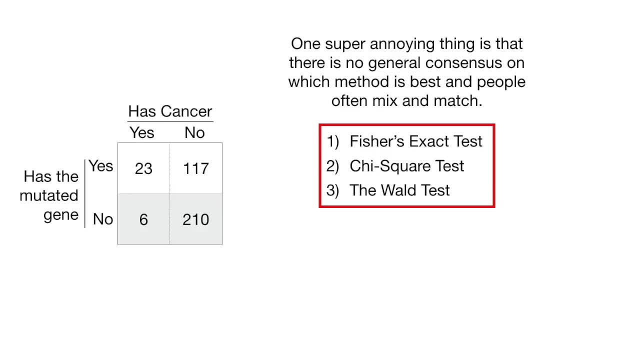 and people often mix and match. One super annoying thing is that there is no general contensis on which method is best and people often mix and match: Fisher's Exact Test, Friedman's Exact Test, Fisher's Exact Test, Er ROM And some people are happy to let Wald do all the work: calculate the p-value and the confidence interval. 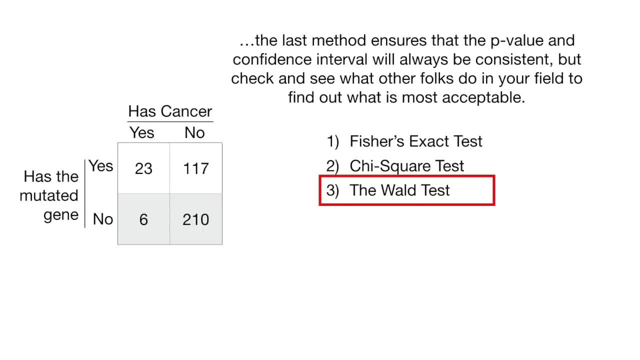 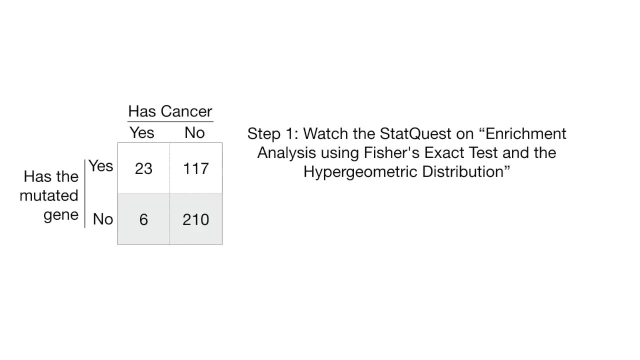 The last method ensures that the p-value and confidence interval will always be consistent. But check and see what other folks do in your field to find out what is most acceptable. So let's start with Fisher's Exact Test, Step 1. Watch the StatQuest on Enrichment Analysis using Fisher's Exact Test and the Hypergeometric Distribution. 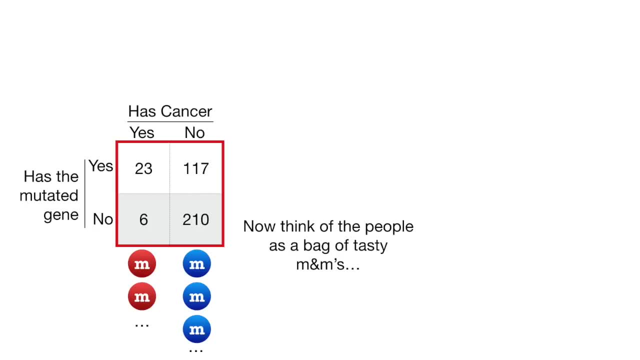 BAM. Now think of the people as a bag of tasty M&M's. People with cancer are represented by 23 plus 6 equals 29 red M&M's. People without cancer are represented by 117 plus 215.. And people with cancer are represented by 310 equals 327. blue M&M's. 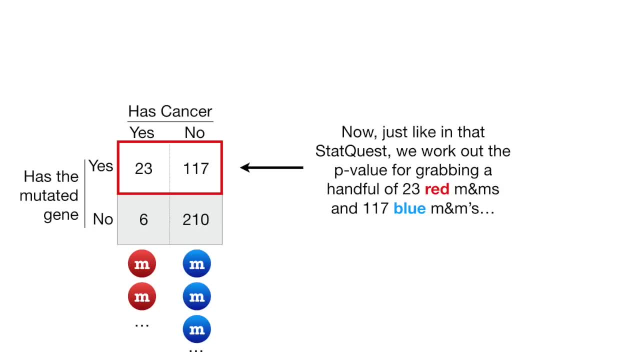 Now, just like in that StatQuest, we work out the p-value for grabbing a handful of 23 red M&M's and 117 blue M&M's. And, just like in that StatQuest, we use a computer and it says the p-value equals 0.00001.. 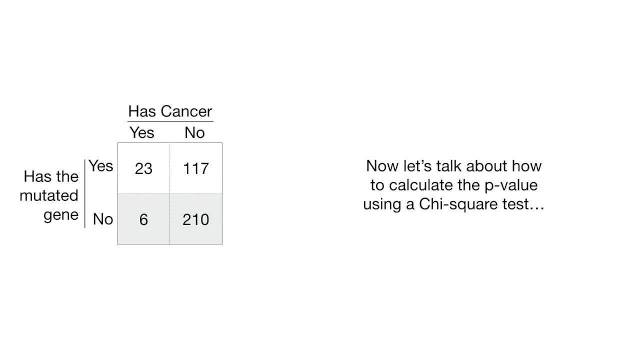 Another small BAM. Now let's talk about how to use the P-Value, How to calculate the P-Value using a Chi-Square test. The Chi-Square test compares the observed values to expected values that assume there is no relationship between the mutated gene and cancer. 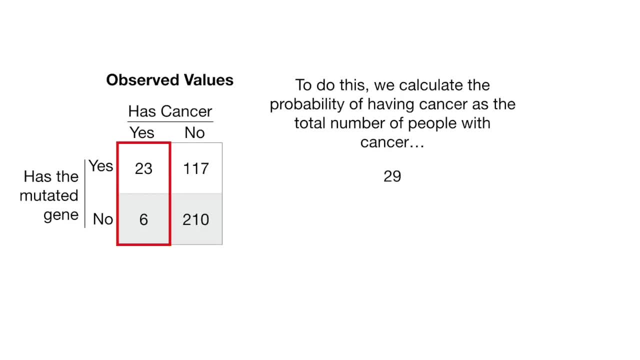 To do this, we calculate the probability of having cancer as the total number of people with cancer, That's 29.. Divided by the total number of people, That's 356.. So the probability of having cancer is 0.08.. 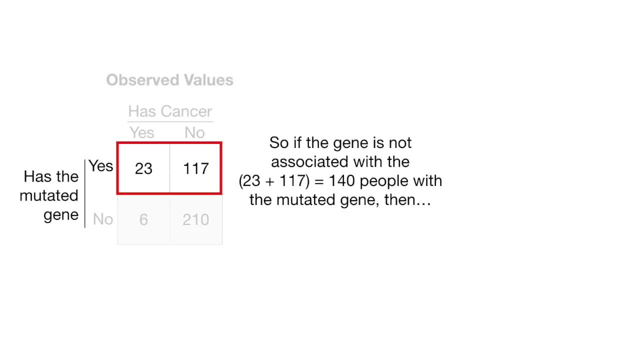 So if the gene is not associated with the 23 plus 117 equals 140 people with the mutated gene. then The probability of having cancer times the number of people with the mutated gene equals 11.2.. Thus, the expected number of people with the mutated gene and cancer. 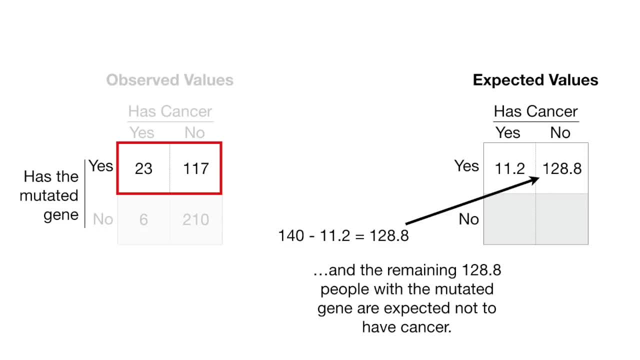 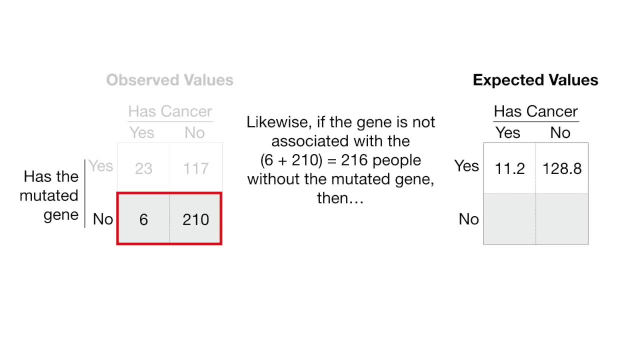 Is 11.2.. And the remaining 128.8 people with the mutated gene are expected not to have cancer. Likewise, if the gene is not associated with the 6 plus 210 equals 216 people without the mutated gene. then 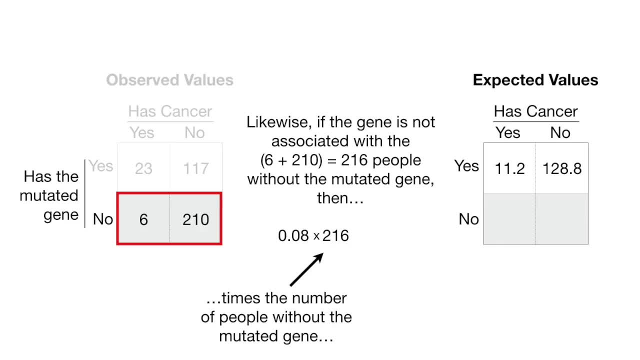 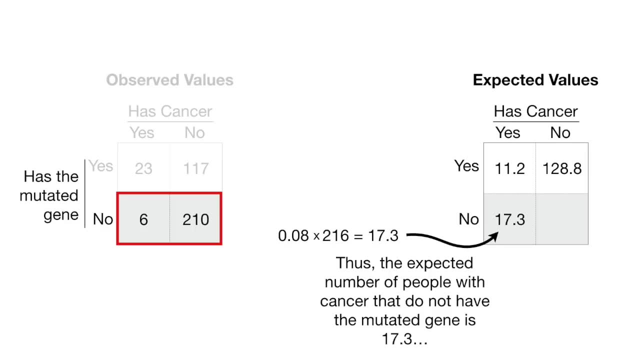 The probability of having cancer Times, the number of people without the mutated gene Equals 17.8.. Thus, the expected number of people with cancer that do not have the mutated gene is 17.3, and the remaining 198.7 people with the mutated gene are expected not to have cancer. 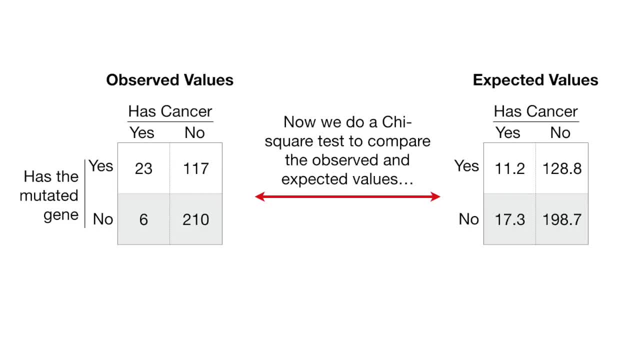 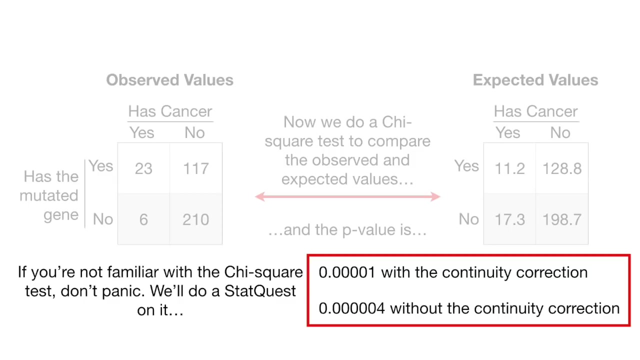 Now we do a chi-square test to compare the observed and expected values, and the p-value is 0.00001 with the continuity correction and 0.00004 without the continuity correction. If you're not familiar with the chi-square test, don't panic, we'll do a stat quest. 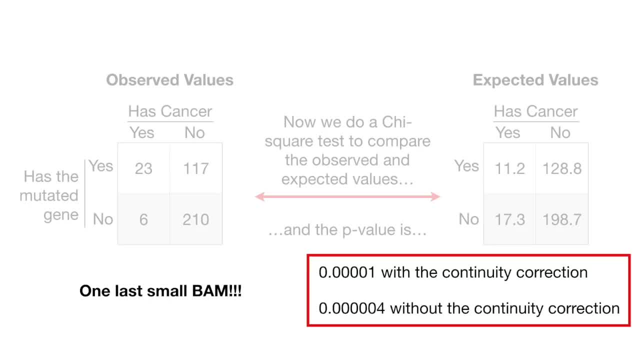 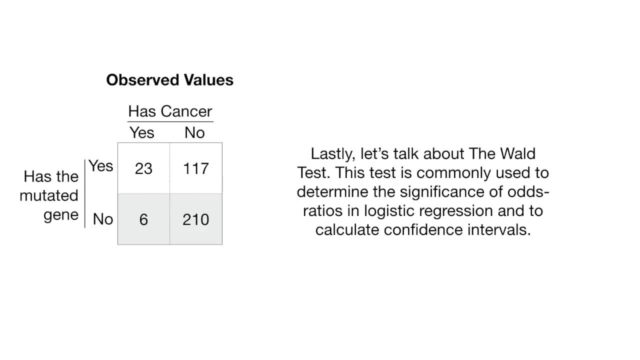 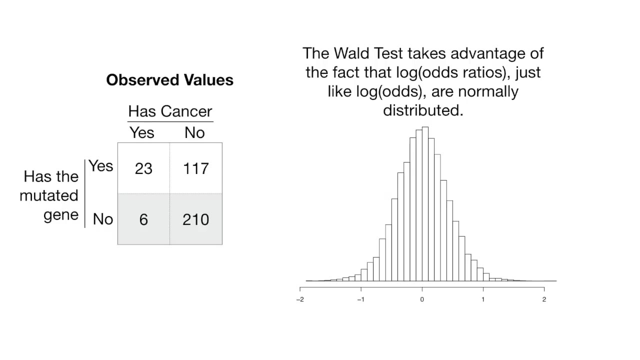 on it One last small bam. Lastly, let's talk about the Wald test. This test is commonly used to determine the significant number of people with cancer that do not have the mutated gene. The Wald test takes advantage of the fact that the log of the odds ratios, just like. 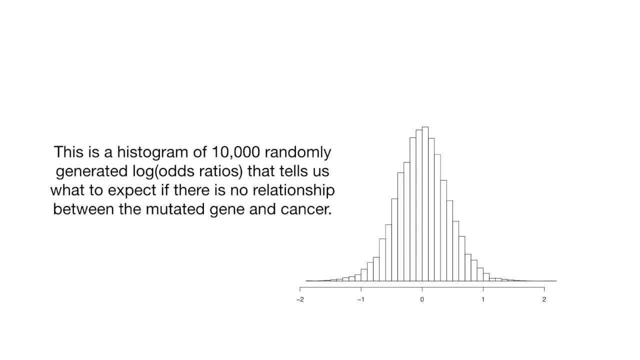 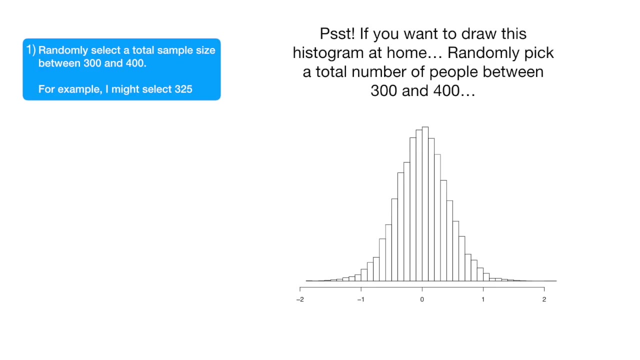 the log of the odds are normally distributed. This is a histogram of 10,000 randomly generated log of the odds ratios that tells us what to expect if there is no relationship between the mutated gene and cancer. Psst, If you want to draw this histogram. 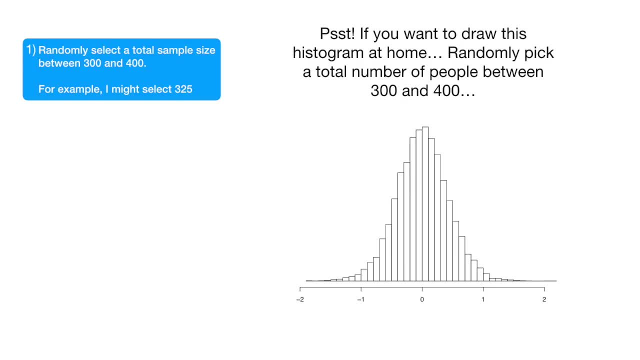 at home. randomly pick a total number of people between 300 and 400.. We do this to simulate the fact that if we repeated this experiment, we might not get the exact same sample size each time. Then, for each sample, select a random number between 0 and 1.. 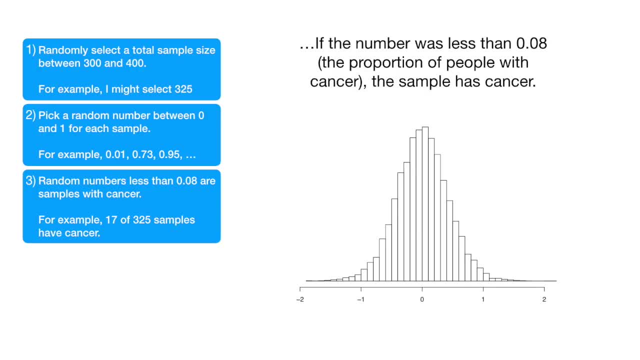 If the number was less than 0.08, the proportion of people with cancer, then the sample has cancer. Then pick another random number and then select another random number between 0 and 1.. If the number was less than 0.39, the proportion of people with the mutated gene, then it has. 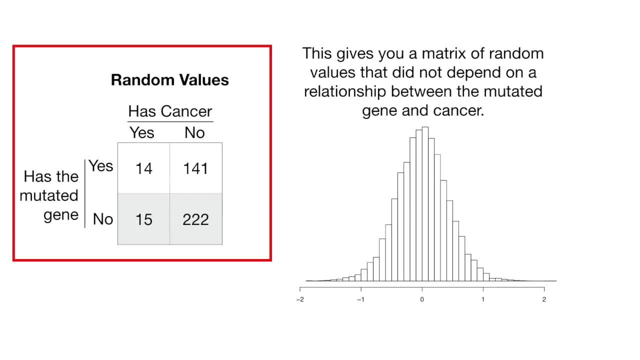 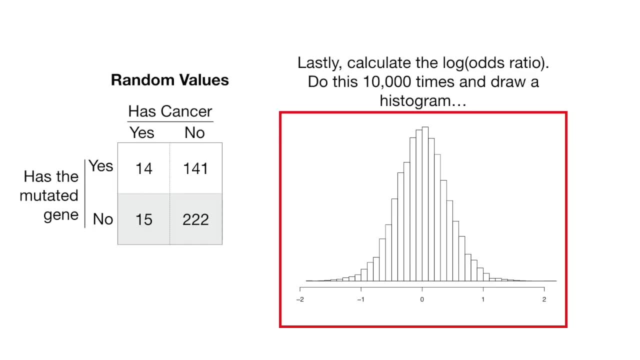 the mutated gene. This gives you a matrix of random values that did not depend on a relationship between the mutated gene and cancer. Lastly, calculate the log of the odds ratio. Do this 10,000 times and draw a histogram- Psst. 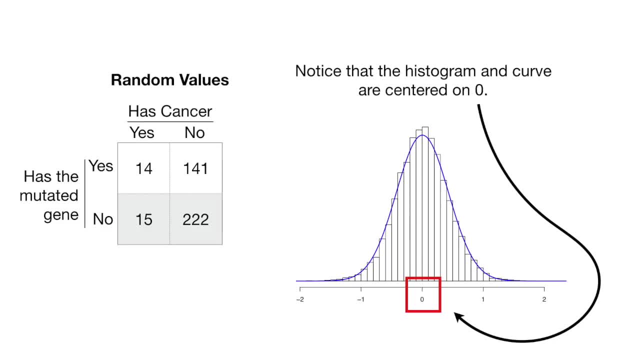 A normal curve fits pretty well. Notice that the histogram and curve are centered on 0.. When there is no difference in the odds, the log of the odds ratio equals 0.. The standard deviation of the 10,000 log of the odds ratios is 0.43.. 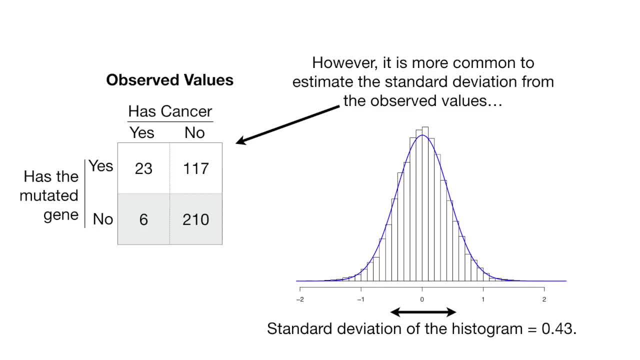 However, it is more common to estimate the standard deviation from the observed values, Psst. You do this by taking the square root of the sum of 1 over each of the observed values. If we do the math, we get 0.47.. 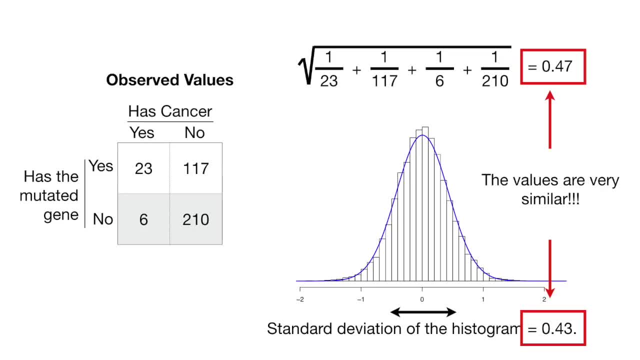 The two different standard deviations that we calculated are very similar. All that the Wald test does is look to see how many standard deviations the observed log of the odds ratio is from 0.. Psst, Psst, Psst, Psst, Psst. 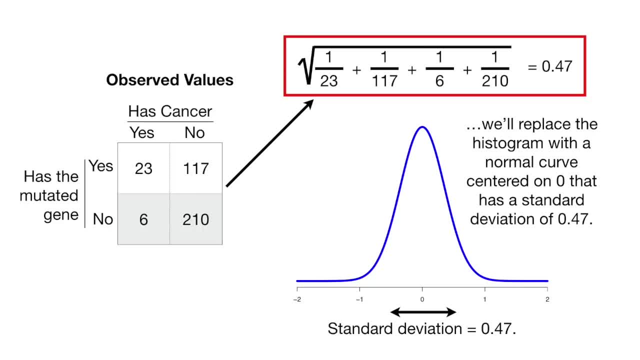 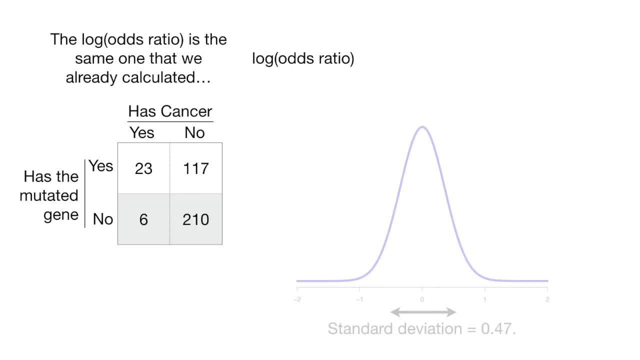 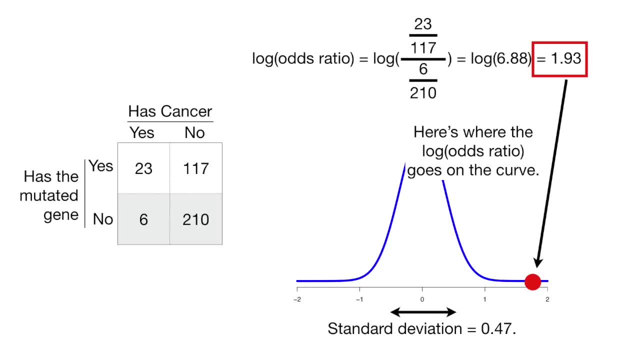 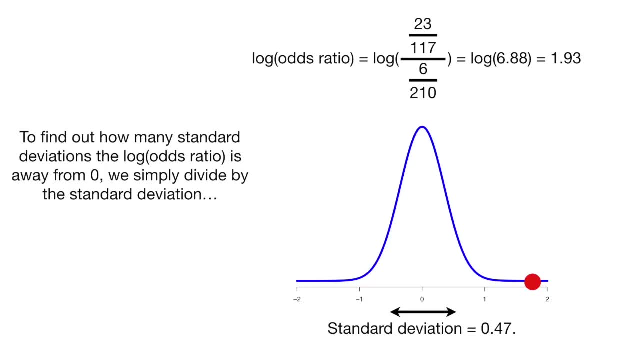 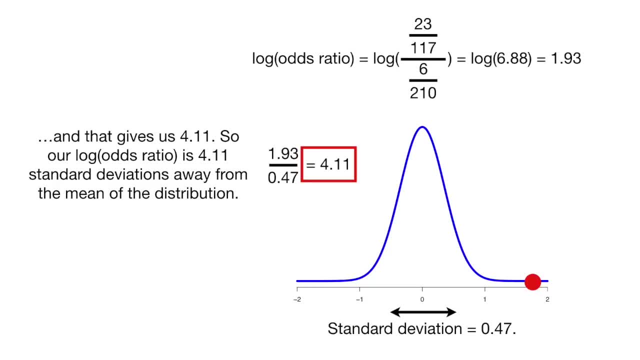 odds ratio is 4.11 standard deviations away from the mean of the distribution. A general rule of thumb with normal distributions is that anything further than two standard deviations from the mean will have a p-value less than 0.05, so we know our log of the odds ratio is statistically. 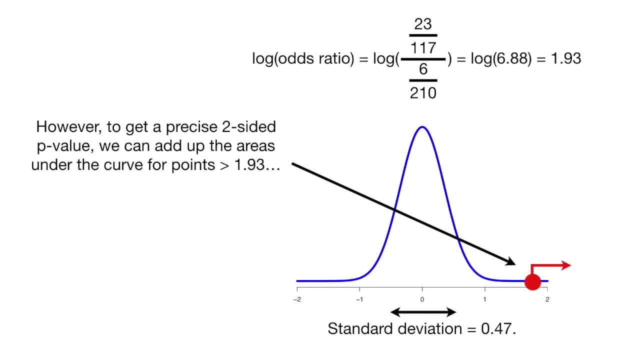 significant. However, to get a precise two-sided p-value, we can add up the areas under the curve for points greater than 1.93 and for points less than negative 1.93.. However, this is traditionally done using a standard normal curve, ie a normal curve that is less than 1.93.. 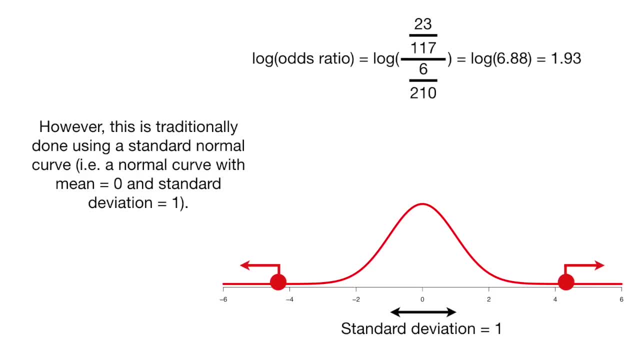 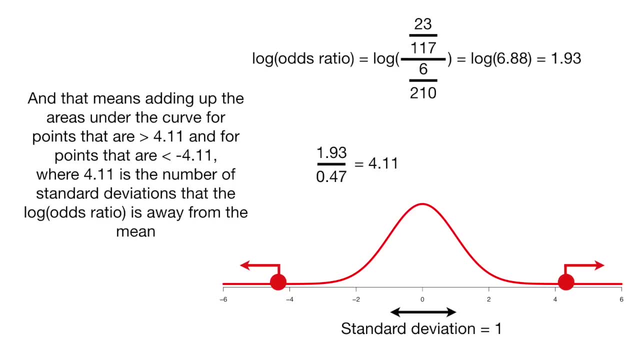 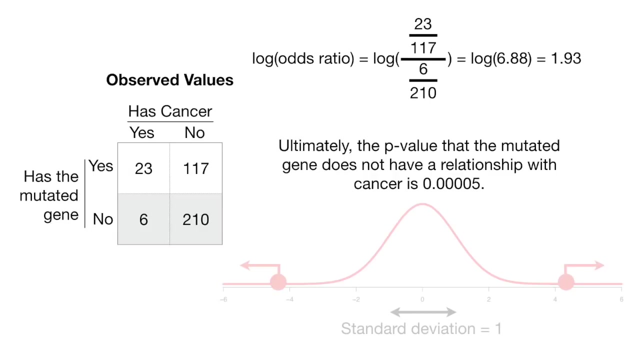 And that means adding up the areas under the curve for points that are greater than 4.11 and for points that are less than negative 4.11, where 4.11 is the number of standard deviations that the log of the odds ratio is away from the mean, Ultimately the p-value that the mutated 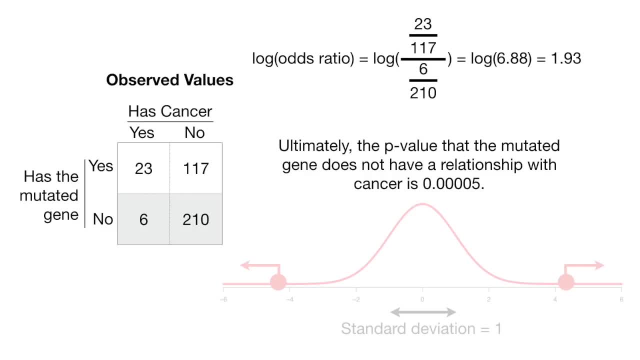 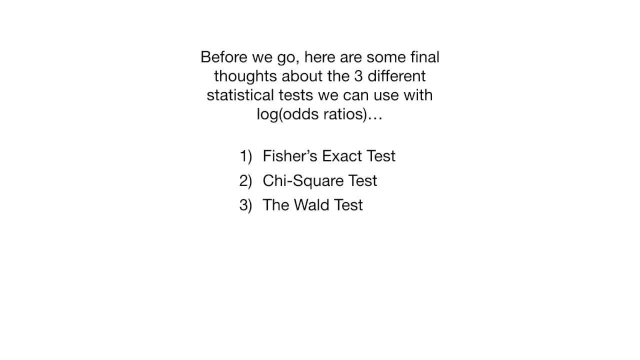 gene does not have a relationship with cancer is 0.01.. So we can add up the areas under the curve for points greater than 1.93 and for points that are less than 0.005.. Double bam. Before we go, here are some final thoughts about the three different statistical tests. 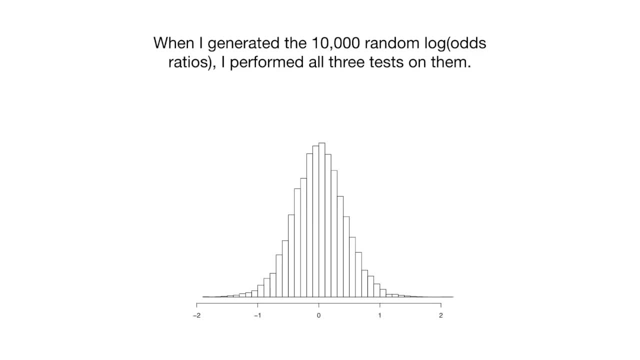 we can use with the log of the odds ratio. When I generated the 10,000 random log of the odds ratios, I performed all three tests on them. If the tests worked as expected, 5% should have p-values less than 0.5.. 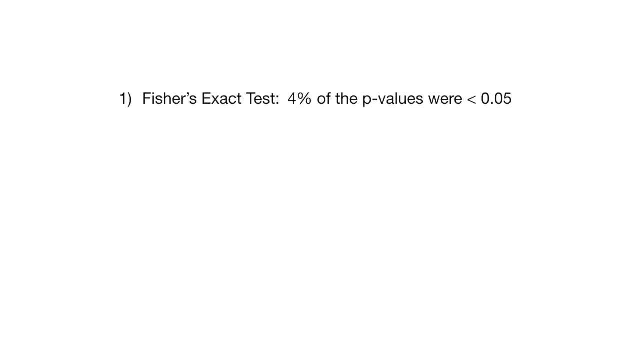 Here's what I got: For Fisher's exact test, 4% of the p-values were less than 0.05.. For the chi-square test, with the continuity correction, 3% of the p-values were less than 0.05.. 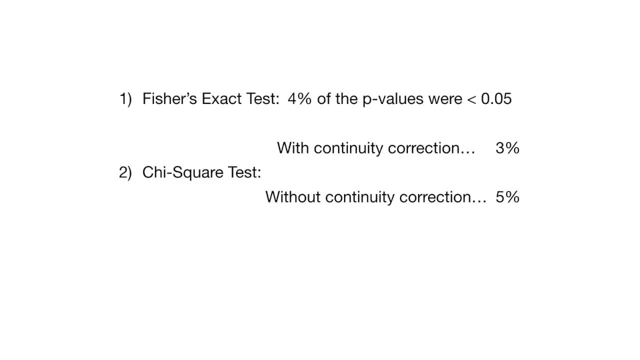 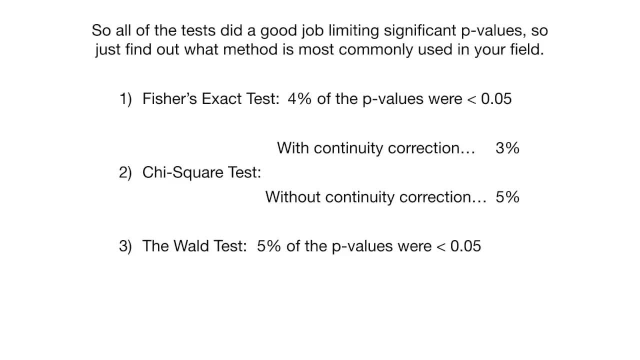 For the Wald test, 5% of the p-values were less than 0.05.. 0.05.. So all of the tests did a good job limiting significant p-values. so just find out what method is most commonly used in your field. Personally, I'd be more comfortable.